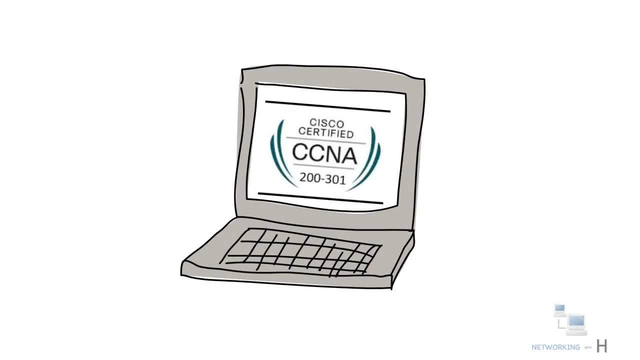 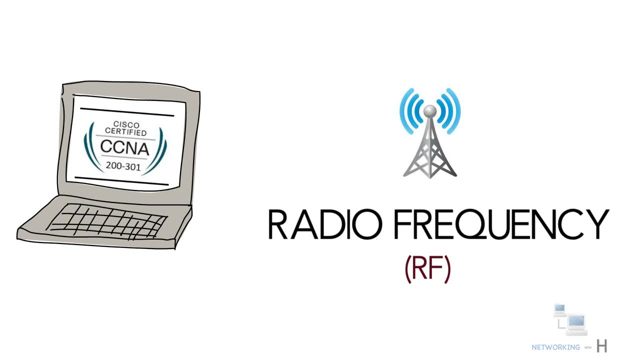 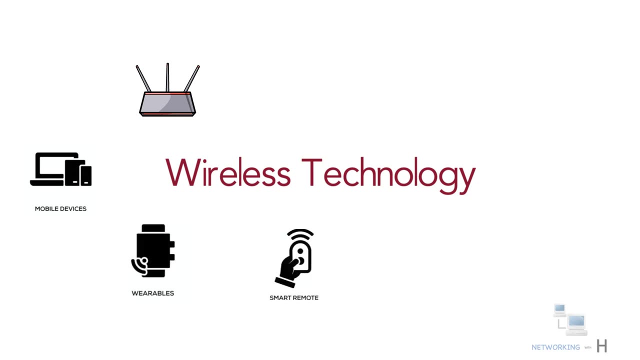 Hello everyone, In this session of CCNA series I'll discuss about radio frequency, also known as RF. Wireless technology is rapidly evolving and is playing an important increasing role in our daily lives throughout the world. Ever thought how those wireless devices communicate with each other? 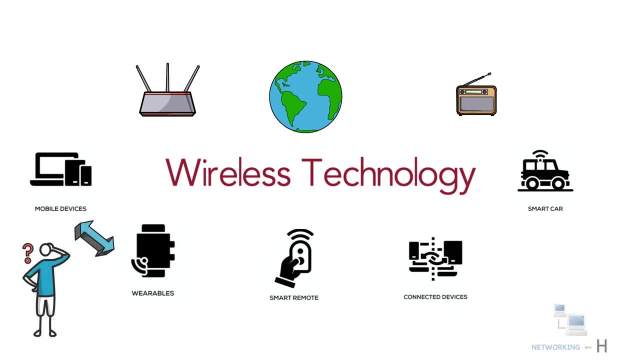 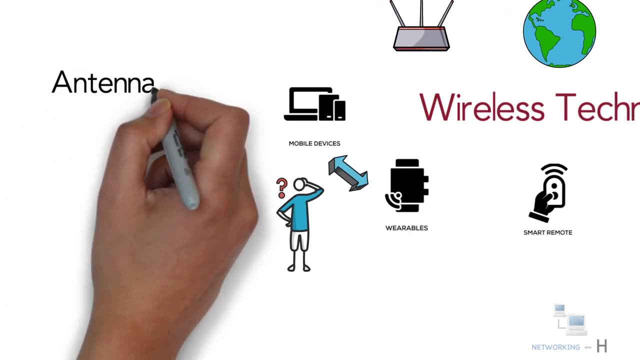 Without any physical medium, like cable, to carry the signal along. Then how does wireless communication transmit signal across the air or free space? The answer is antenna. Every wireless devices are equipped with antennas. Antenna is responsible for the transmission and reception of signal on such devices. 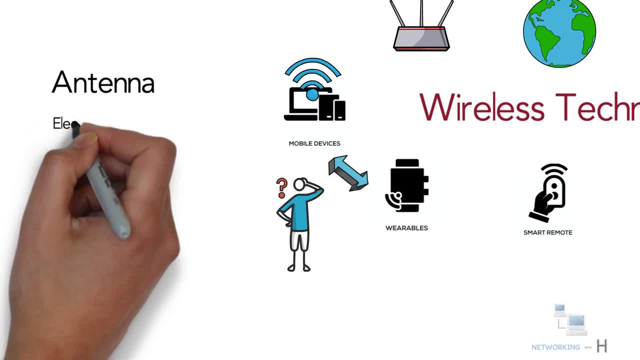 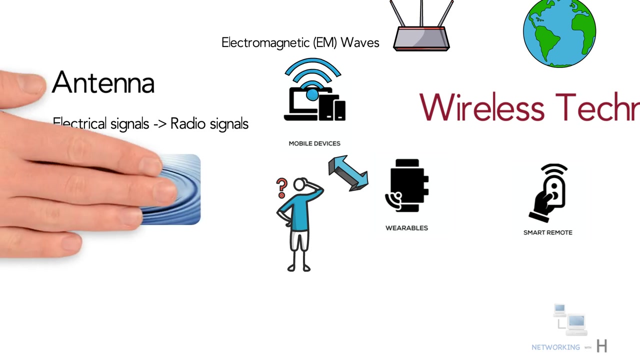 Antennas are electrical devices that transfer. They transform the electrical signals to radio signals in the form of electromagnetic waves. Electromagnetic waves do not travel in straight line. Instead, they travel by expanding in all directions away from the antenna. To get a visual image. think of dropping a pebble into a pond when the surface is still 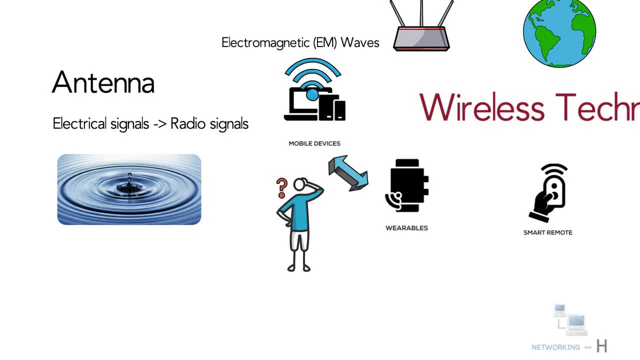 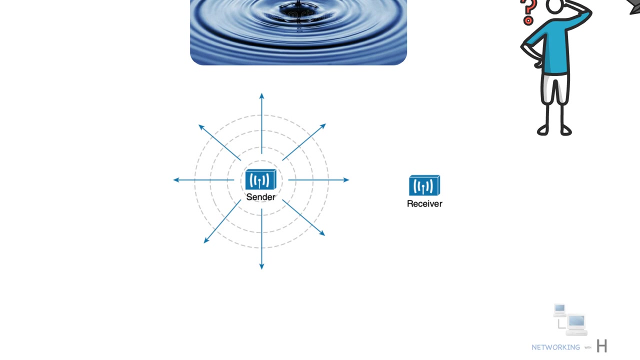 Where it drops in, the pebble sets the water surface in place. The waves that result begin small and expand outward, only to be replaced by new waves. In a free space, the electromagnetic waves expand outward in a similar way. You can take an example of a simple, idealistic antenna that is a single point at the end of a wire. 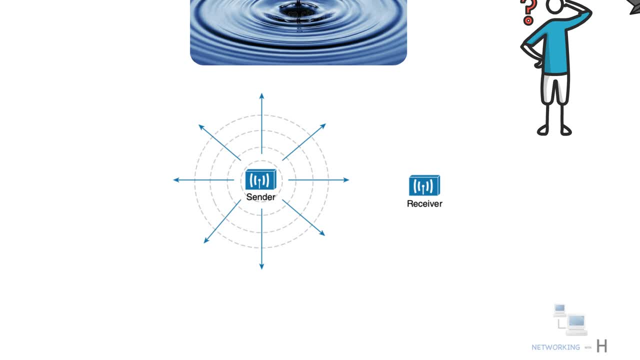 The waves produced expand outward in a spherical shape. The waves will eventually reach the receiver At the receiving end of a wireless link. the process is reversed: As the electromagnetic waves reach the receiver's antenna, they induce an electrical signal. If everything works right, the received signal will be a reasonable copy of the original transmitted signal. 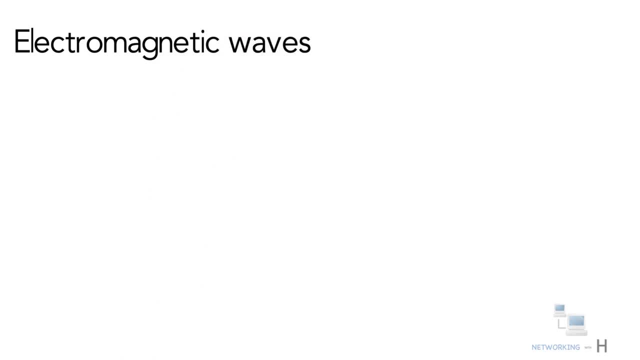 Electromagnetic waves are measured using frequency. Frequency is equal to number of cycles per second. That is number of times the signal makes one complete up and down cycle in one second. A cycle can begin as the signal rises from the center line, falls through the center line and rises again to meet the center line.